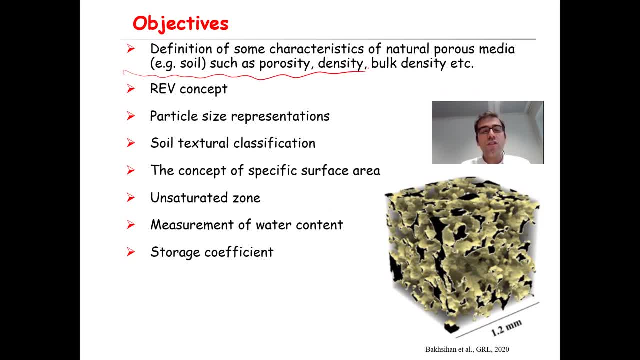 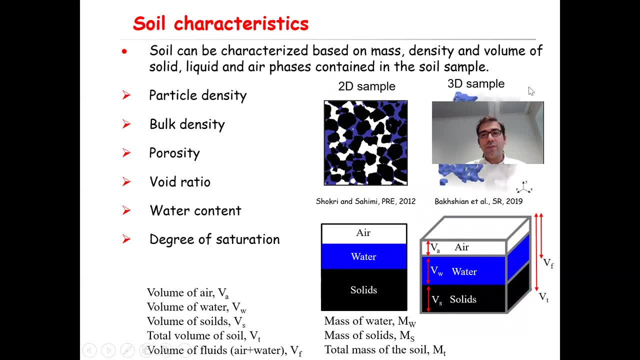 first item and in future videos which will be uploaded to this channel, we will cover other part of this chapter. Okay, so soil characteristics. So soil can be characterized based on the mass, density and volume of solid liquid and air faces contained in the soil sample. So what do I mean by? 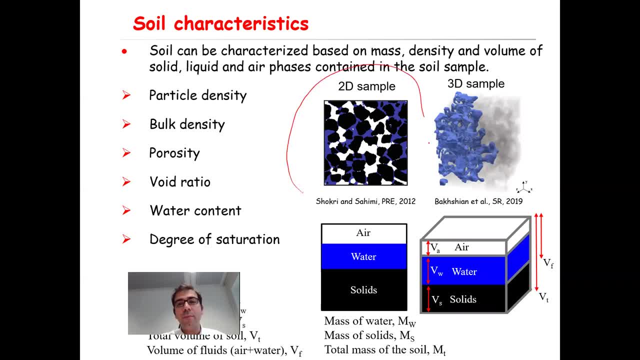 that. So look at, for example, here it's a 2D sample. okay, this is again another results from our another results from our group, which was published in 2012.. Here you see, the black color is the sand grain, I believe the picture. this picture was captured by synchrotron X-ray tomography. 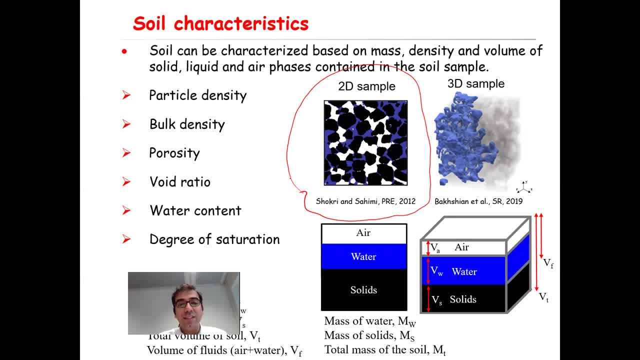 and which enabled us basically to look into the phase distribution in sand in sanding material which was on the drying process. In any case, this picture- the black color is the sand grains, the blue color is the liquid phase and or water, and the white color is the air phase. okay, Or you can as well consider 3D sample this: 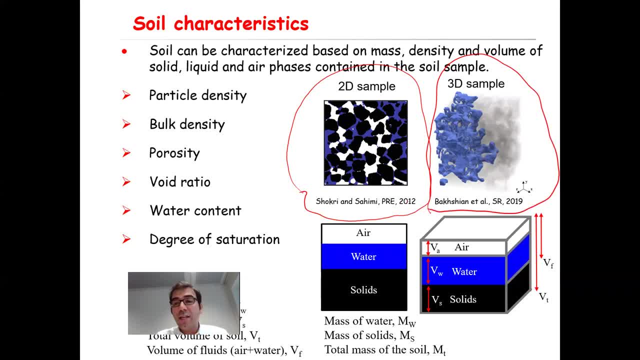 This was again our own results. It was published in 2019 in Scientific Report. Here, by simulation, we look into the fluid displacement in 3D rock samples. The blue color is the fluid and the gray color is the rock sample. 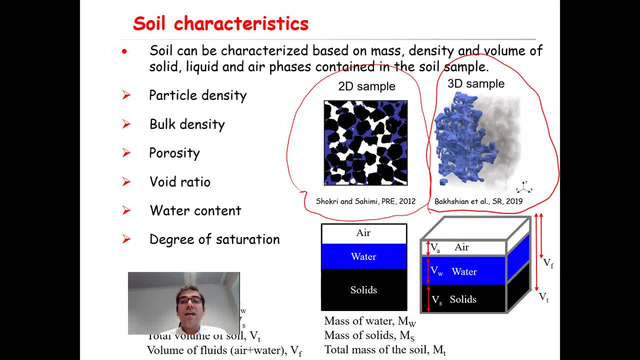 Okay, so you have here a solid phase, that is, the rock, the liquid phase and the gas phase or air phase. Okay, so you can represent, or you can partition this volume into something like that. You say: okay, Vs, that is, represent the volume of the solid, that's this part of this volume. 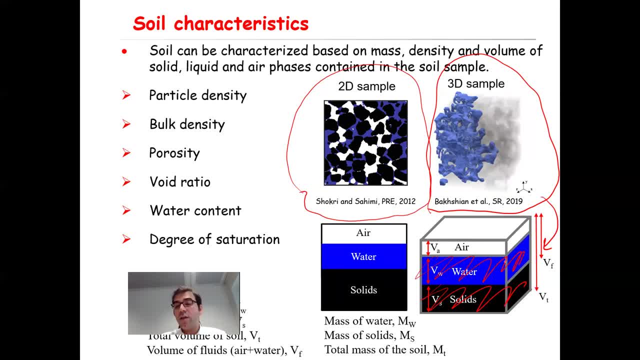 Another part is the liquid phase. let's call it water, okay, but it could be anything else, And then you have as well Va. that is the air phase, okay. So that sentence I said at top, depending on the basically relationship between this Va, Vw, Vs. 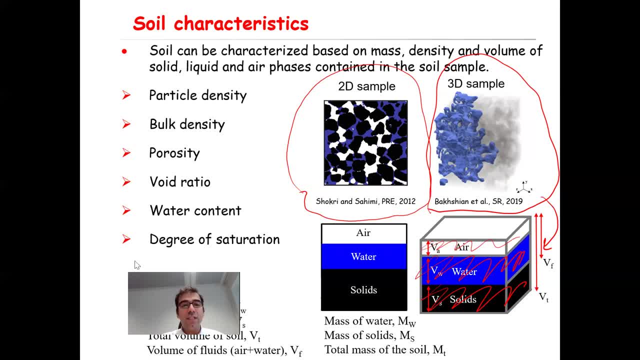 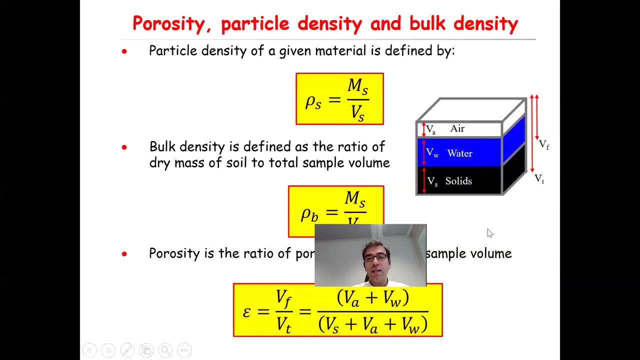 and also the mass of different phases. you can define different properties of this porous medium, including particle density, bulk Density, porosity, void ratio, water content and degree of saturation. okay, And we wanted to cover these definitions in this video today. 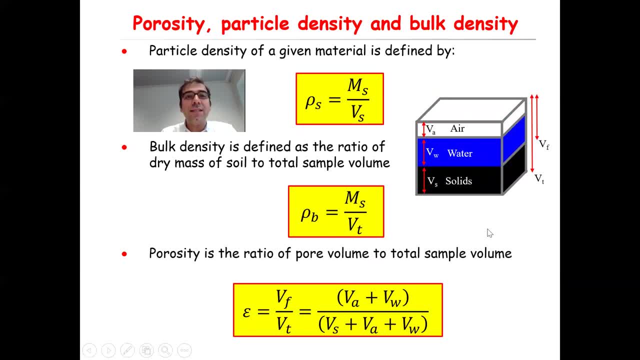 Okay, so first let's start with particle density. Particle density or density of the solid phase of a given material is defined by rho s, that is the particle density, or solid phase. Density divided is equal to ms, that is the mass of the solid 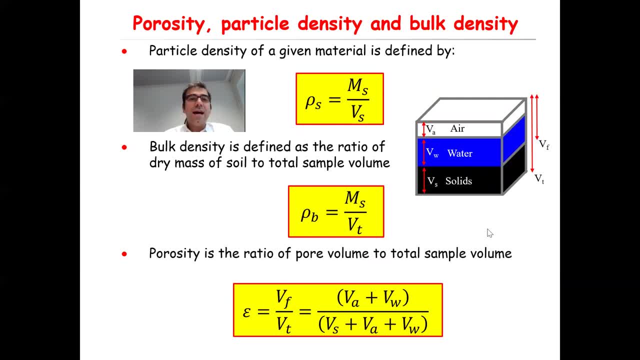 divided by the mass of the solid Density, divided by Vs, that is the volume of the solid. okay, Another quantity is bulk. density is defined as the ratio of dry mass of soil. okay, What do I mean by dry mass of soil? 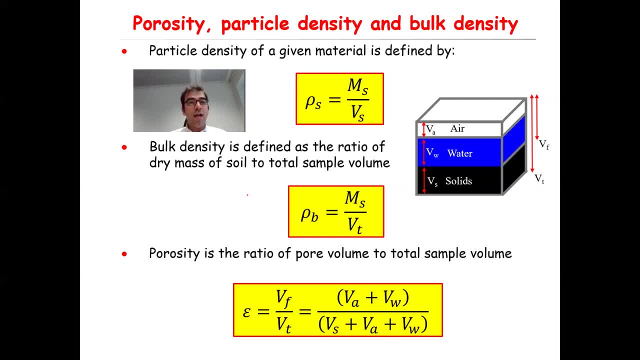 That means, let's say, if you have wet soil, you put it in the oven, you dry it and then you put it on a balance. you measure the weight. okay, That will be the dry mass of soil divided by the total sample volume. 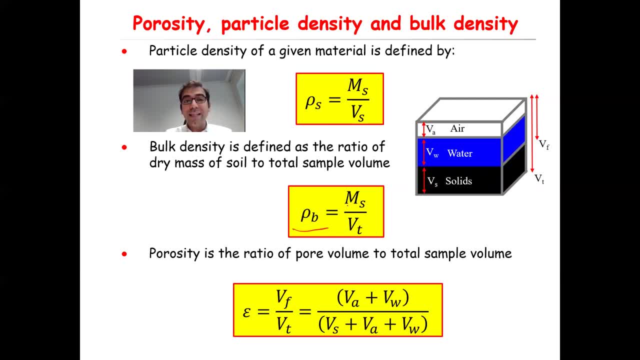 So rho b, that is the bulk density, is equal to ms, that is, the dry mass of soil divided by the total volume, that is the Vt Total volume. Total volume is equal to, basically, Vs plus Vw plus Va. okay, 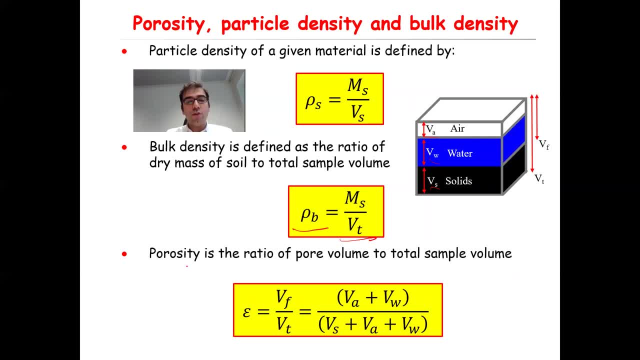 So porosity, which is an important characteristic of a porous medium, of a porous medium, is defined as the ratio of the pore volume- okay- to total sample volume. So epsilon, that is the porosity, is equal to Vf, that is the volume of the basically fluid. 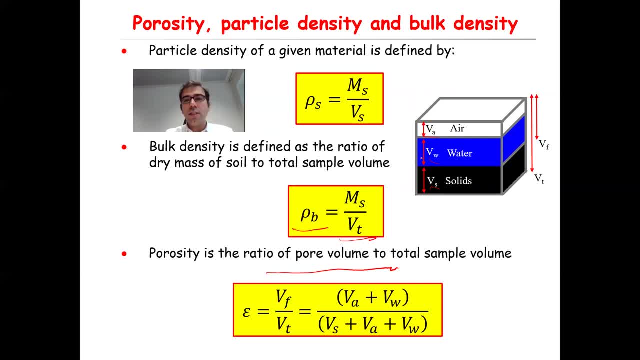 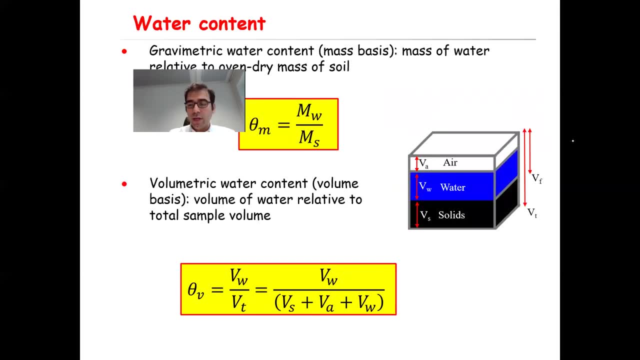 because they're here- or the water, Vw plus Va. air. The air and water summation of the volume will be equal to Vf. okay, So Va plus Vw divided by Vtotal, which is equal to Vs plus Vw plus Va. 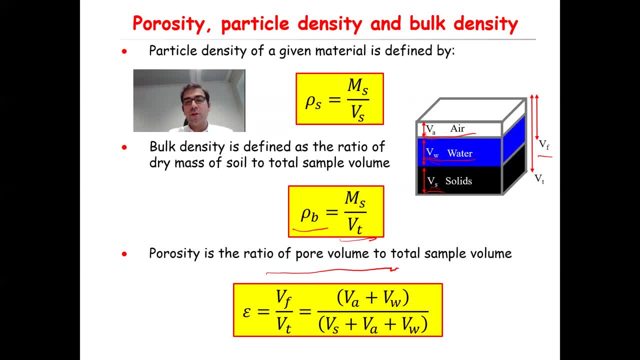 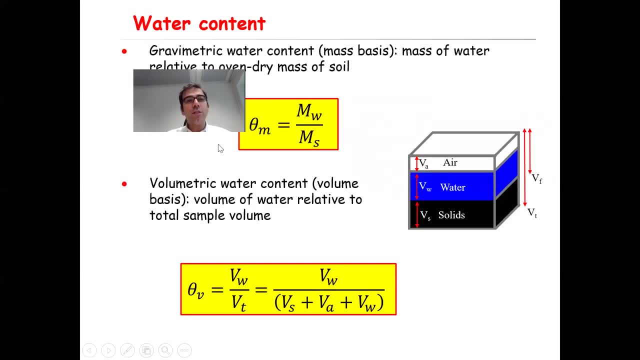 So porosity is equal to Vf divided by Vt, equal to Va plus Vw divided by Vs plus Va plus Vw. okay, Another important quantity is water content. And water content you can measure. you can present it in two ways: gravimetric water content or mass-based water content. 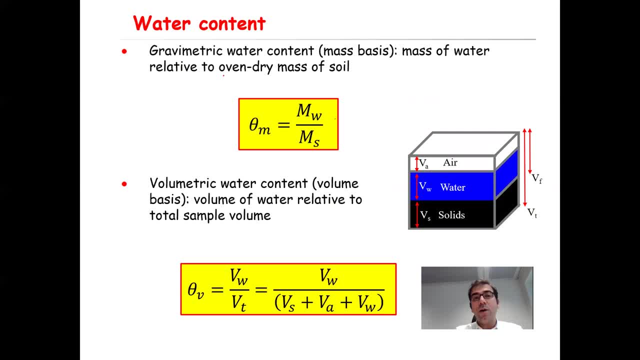 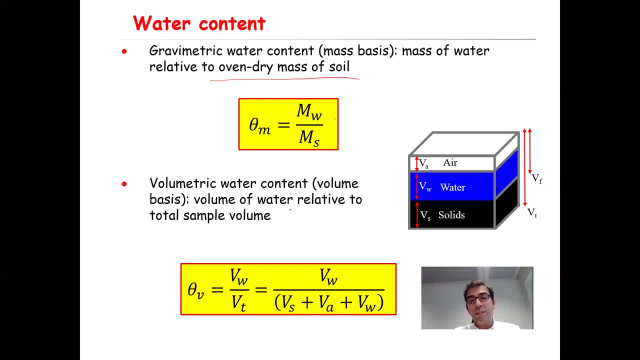 And another way of presenting water content is volumetric water content. theta V, that is volume of water Vw divided by the total volume, And total volume is Vs plus Va plus Vw. So theta M and theta V, gravimetric water content and volumetric water content- okay, 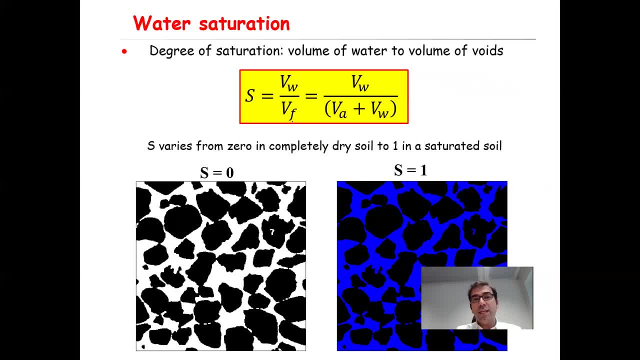 And there is another quantity called water saturation, That, or degree of saturation, which is the volume of water to volume of void, okay, or volume of the fluid, basically, which is air and water, right, So that will be Vw, that is, volume of water divided volume of void, or volume of fluid, which is Vf, which is equal to Va plus Vw. 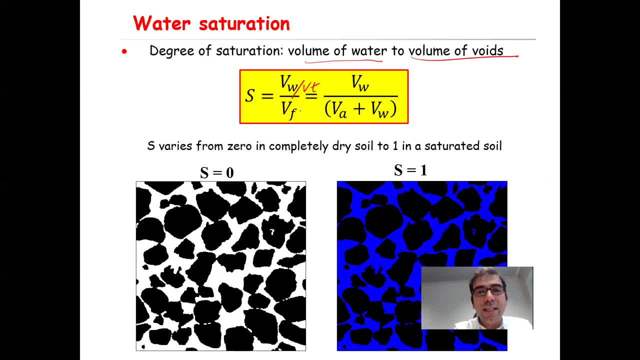 Here. if you divide everything by Vt, that is the total volume, right, you get Vw divided by Vt is equal to theta V. That is the definition of the volumetric. Okay, Okay, Volumetric water content divided by Vf, divided by Vt, that's the definition of the porosity. 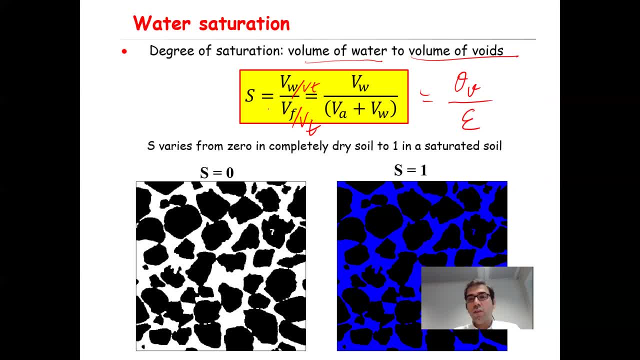 So you already derived another equation, That is, saturation is equal to the volumetric water content divided by porosity. Okay, And as you can see here in this equation, the saturation, the value of the saturation, varies from zero in a completely dry sample to one in a saturated soil. 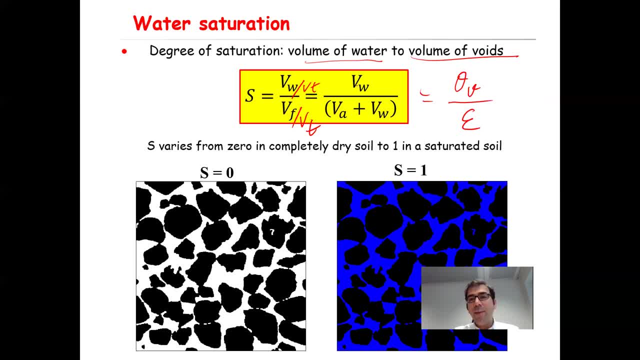 Why? Because here, you see here, if the Vw is equal to zero, right, the saturation will be zero. And so this is like you see here, the black color is the sand grain, the white color is the air phase. there is no liquid phase. that means Vw is equal to zero. the system is completely dry. and when the system is completely dry, Vw is equal to zero. therefore, saturation is equal to zero. 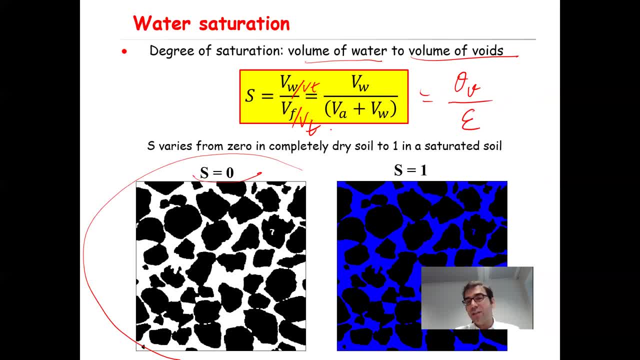 On the other hand, if Va is equal to zero, right, if there is no air in the system, so Vw divided by Vw, basically, will be equal to one, and that's the maximum, The maximum volume, maximum value of the saturation, which is this example. 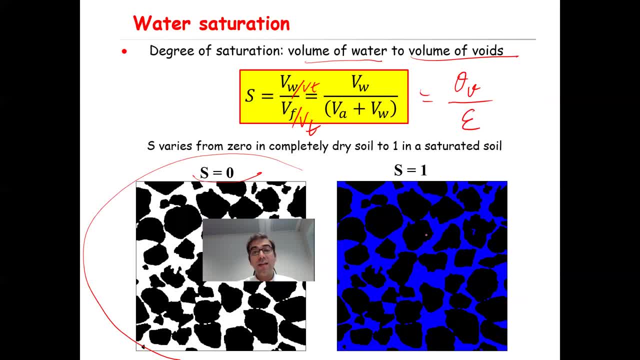 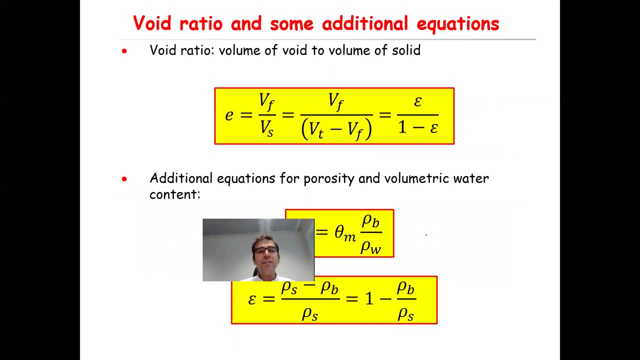 You see here, the blue color is the liquid phase and the black color is the solid phase. So therefore, the saturation values ranges from zero to one in the case of completely dry to fully saturated system respectively. Okay, Another definition is the void ratio, and void ratio is defined as the volume of the void volume or volume of the fluid. 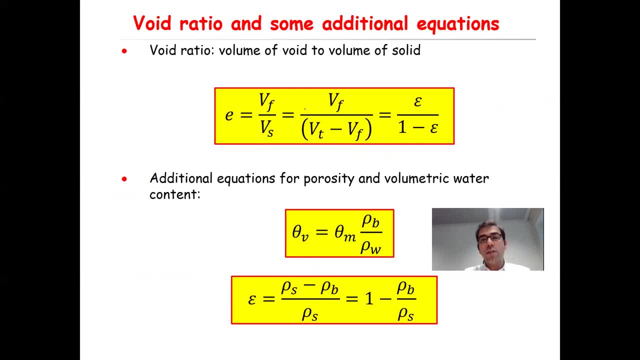 Okay, So Vw divided by Vs, that is volume of the solid. so in other words you can write: Vf divided by volume of solid is equal to total volume minus volume of fluid right. And if now you divide everything by Vt, right, so Vf divided by Vt will be definition of porosity. Vt divided by Vt is one. Vf divided by Vt is epsilon. 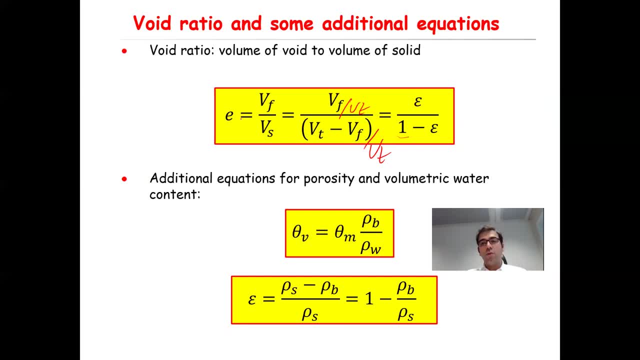 So porosity divided by one minus porosity will be equal to void ratio. Okay, So using these basic equations you can derive additional equations. For example, you can derive theta V, that is, the volumetric water content is equal to gravimetric water content times rho B divided by rho W. 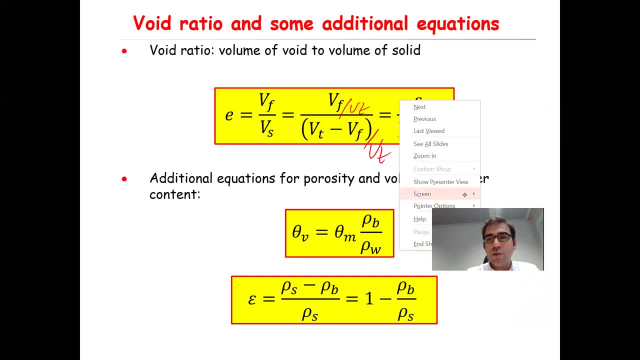 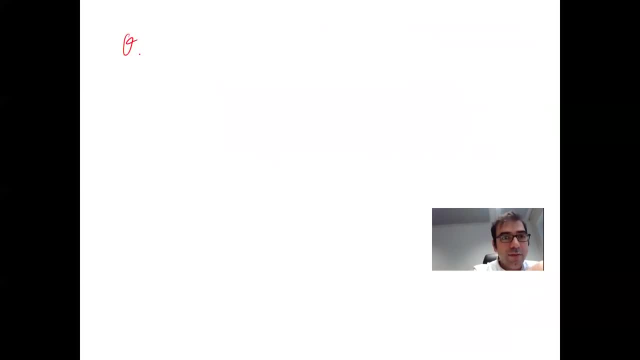 In fact, you can derive this equation yourself. Let me see if I can. yeah, I can. this runs now. So the equation is: theta V is equal to theta M times rho B divided by rho W. Okay, So how can you derive this equation? 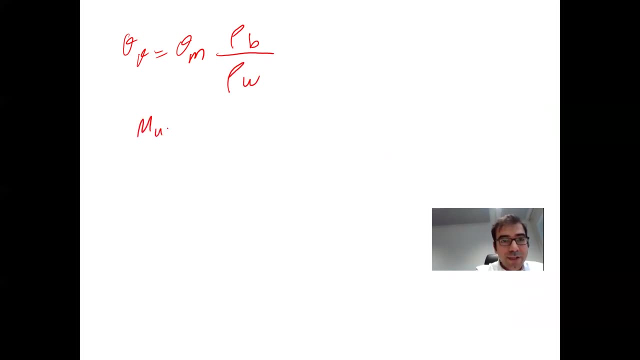 So here in a sense. So if you have a mass of theta M, we know theta M is equal to mass of water divided by mass of solid. Okay, That's a definition of the gravimetric water content times. rho B, that is a bulk density which is equal to mass of solid divided by total volume. 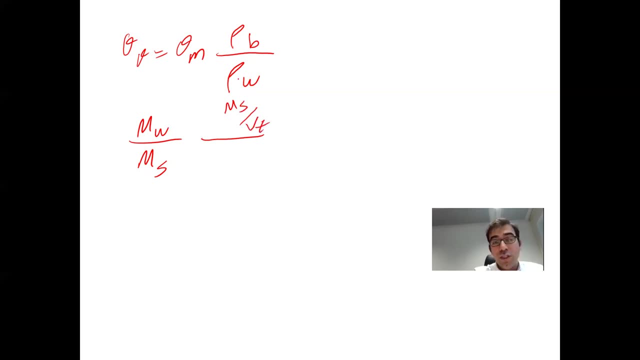 You already have it in your slide. divided by rho W, which is the density of water, which is mass of water divided by volume of water. Okay, And that will be equal to Mw right. divided by Ms times- Ms at top this times, this Vw. divided by Vt times Mw. 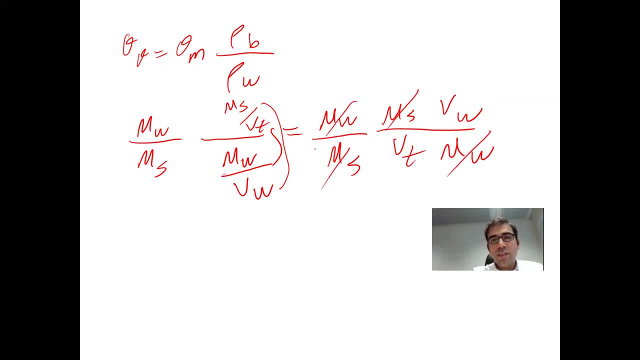 Okay, So here Ms is out, Mw is out. So that is equal to Vw divided by Vt, And by definition this is equal to theta V, if you look at your slides Right. So basically we showed here that the theta M times rho B divided by rho W is equal to theta V. 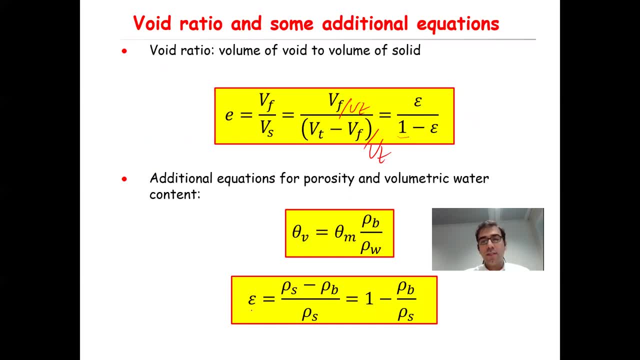 Okay, There is another equation. for example you can write: porosity is equal to rho S minus rho B divided by rho S. that is the, that is, the density of the solid minus bulk density, divided by, basically, the density of the solid phase or particle density, which is equal to one rho S divided by rho S, is one rho B minus rho B divided by rho S. 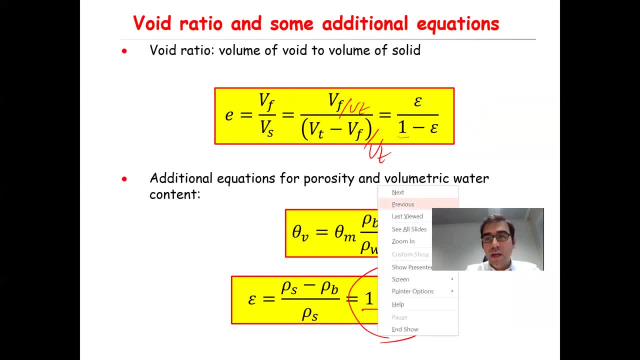 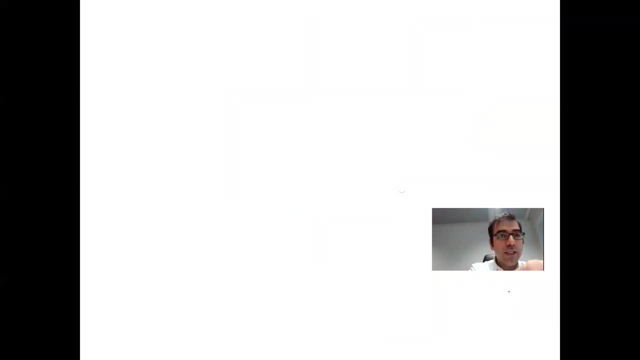 You can as well derive this equation yourself, So here I can show it to you how to do that. I can show how to do that. So here the equation is: Porosity is equal to one minus rho B divided by rho S. Okay, 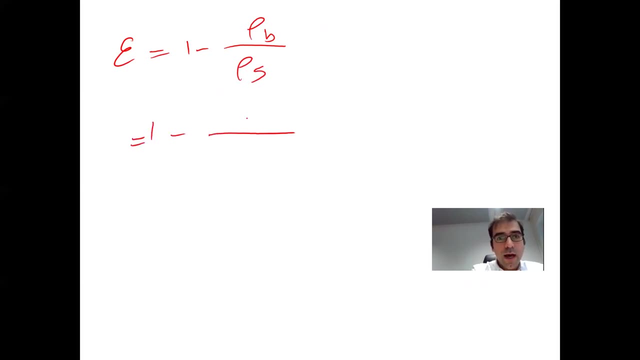 So that one you can write here one minus. instead of rho B, I write Ms divided by Vt, that's the definition of the bulk density divided by. instead of rho S, I write Ms divided by volume of the solid, that is Vs. 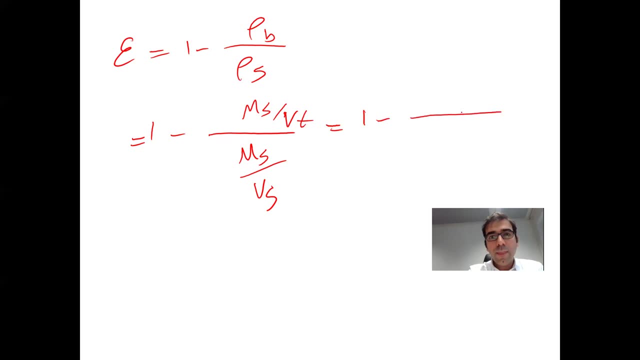 Okay, So that will be equal to one minus. okay, Ms times Vs. That is Ms, So Ms is out here. therefore, this one will be equal to one minus Vs. divided by Vt, which is equal to Vt, that will be Vt minus Vs, okay. 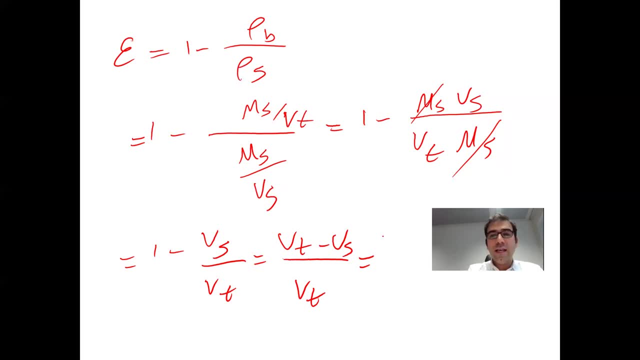 So the total volume minus volume of the solid phase, that gives you volume of the fluid or void volume, Vf divided by Vt And by definition, if you look at the previous slide- the previous slide- you'll see Vf divided by Vt is different. 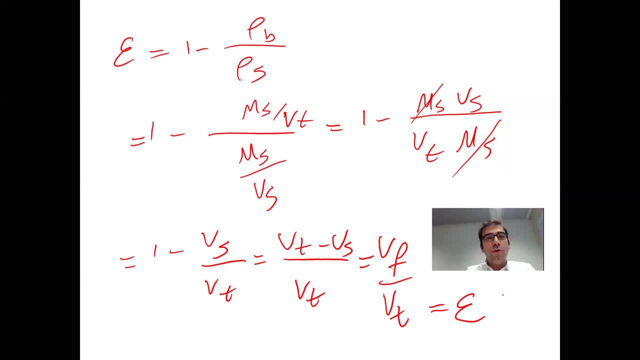 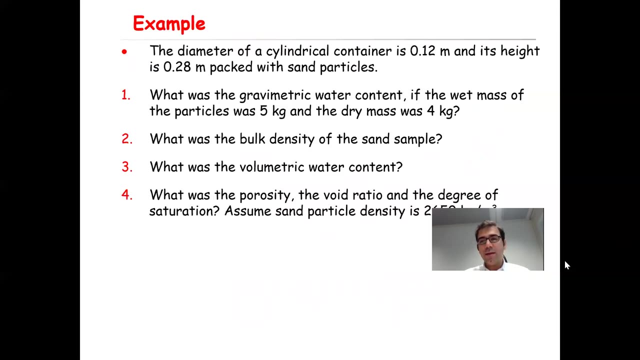 So the total volume of the solid phase is the same as one minus rho B divided by rho S. Okay, So therefore you here. you prove porosity is equal to one minus rho B divided by rho S. Okay, So now there's an example here. 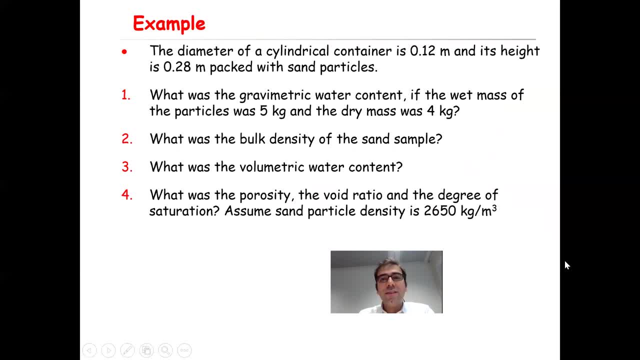 Let's solve this example. Example is: the diameter of a cylindrical container is 0.12 meter and its height is 0.28 meter, packed with sand particles. Okay, So you have a cylindrical container packed with sand particles and you have the diamond of the cylinder. 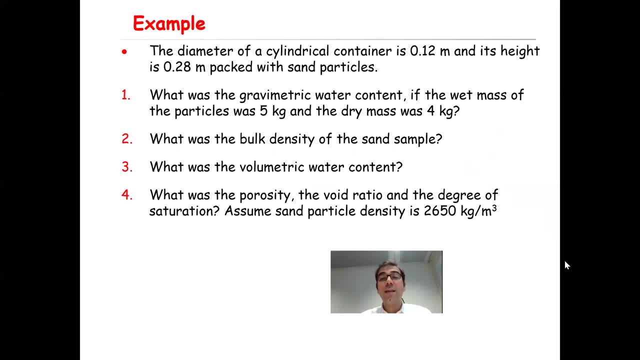 So the question has four parts. The first is: do you have an empty cylinder Or do you have a solid cylinder? first part is: what was the gravimetric water content if the wet mass of the particles was was five kilo a kilogram and the dry mass was four kilogram? so you have the wet mass. 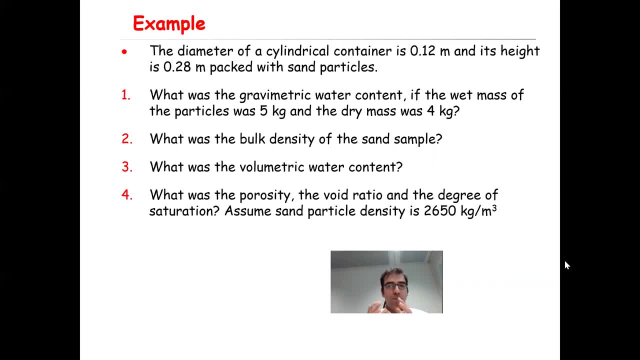 imagine you put that in the oven and then you dry it. you measure it again. that now is four kilo. the question is: what is the gravimetric water, gravimetric water content? and another part of the question is what was the bulk density of the sand sample? another one is: what's the volumetric? 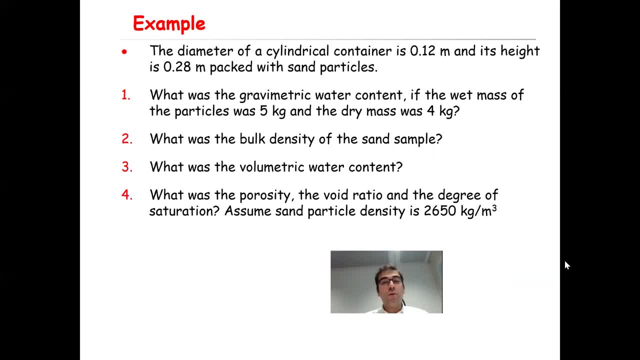 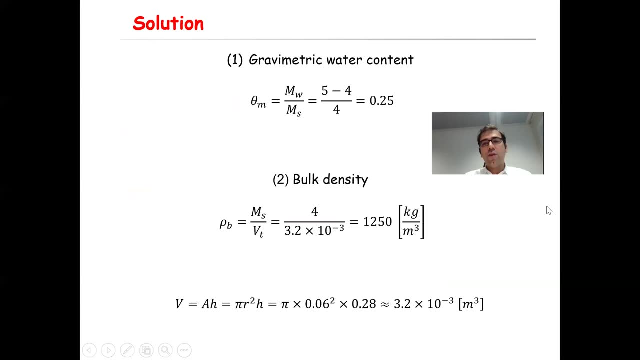 water content. and then the last part of the question is: what's the porosity, what's the void ratio, what's the degree of saturation? and assume sand particle density is 2650 kilogram per cubic meter. okay, so let's first solve the first part of the question, that was: 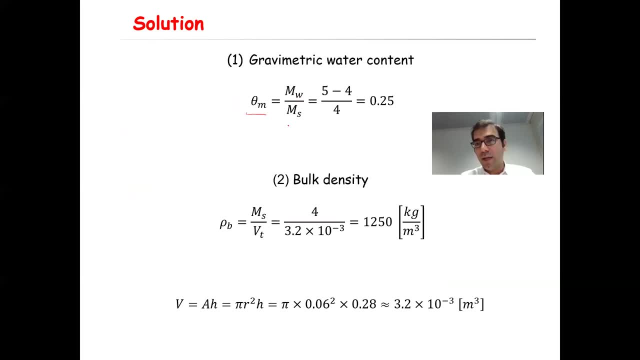 gravimetric water content, which is equal to mw divided by ms. you have this equation. so mass of the water, so the wet mass of the soil or sand particle was five kilogram. The dry mass was 4 kg. Therefore, the mass of the water is 5 minus 4,. 5 minus 4, divided by ms, that is 4.. 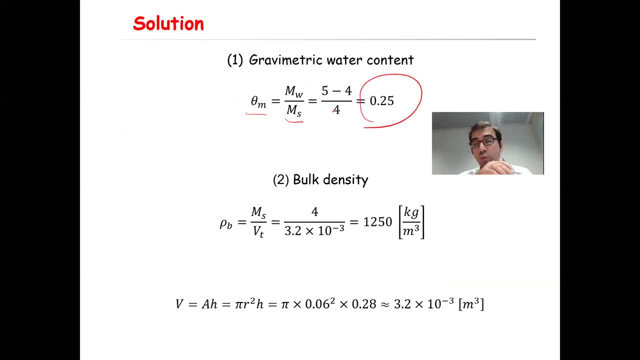 So that will be 1 divided by 4, which will be 25% or 0.25.. That will be the geometric water content. Another part of the question was about bulk density And rho b we know is equal to ms divided by vt. 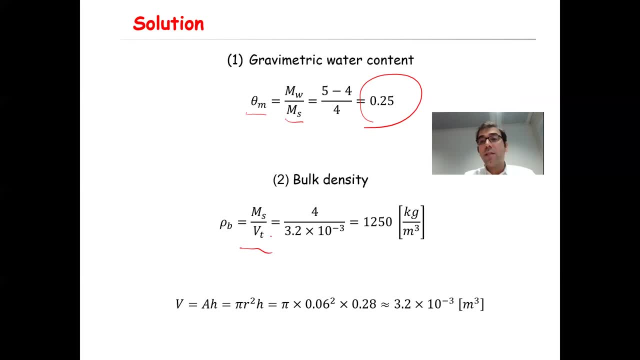 ms is the mass of the solid, that is, 4 kg, divided by the total volume, okay, And the total volume of the sample. so you know it is a cylindrical sample. okay, You have the height given in the question and you have the diameter: 2r. 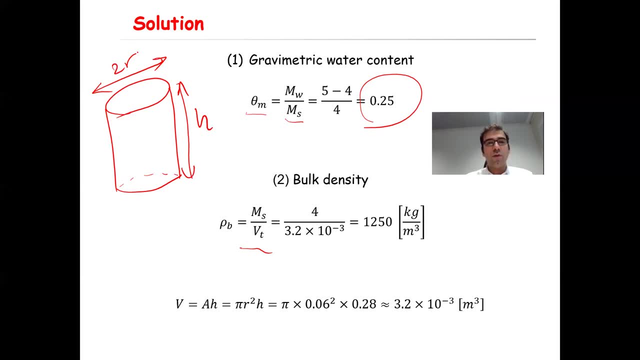 r is the radius and you have it in the question. It's given in the question. so v is equal to a times h, That is a. the area is pi r squared times the height, which will be equal to pi times. 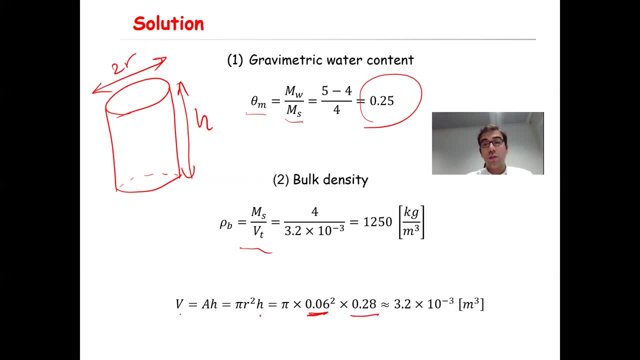 this is given in the question and the height has been given in the question. So the total, or the volume of that sample, or total volume, is equal to 3.2 times 10, to the minus 3 cubic meter and that will be your vt. okay, total volume, okay. 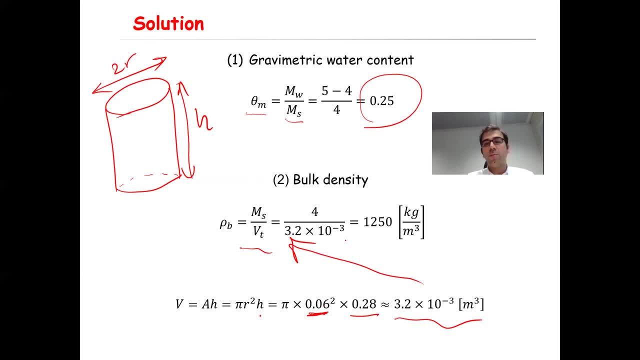 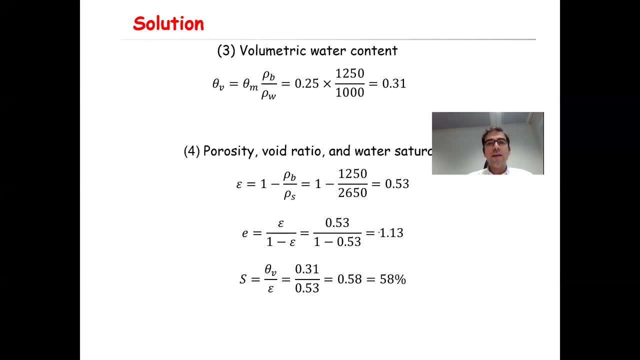 So that will be. rho b is equal to 4 divided by 3.2 times 10, to the minus 3, which will be equal to 1250 kg per cubic meter. So that is the bulk density. The third part of the question was about 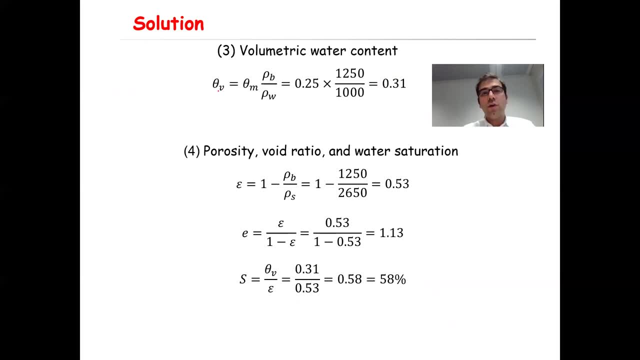 volumetric water content. and for the volumetric water content you have, theta v is equal to theta m. that is the gravimetric water content times, rho b divided by rho w. So gravimetric water content you already calculated. 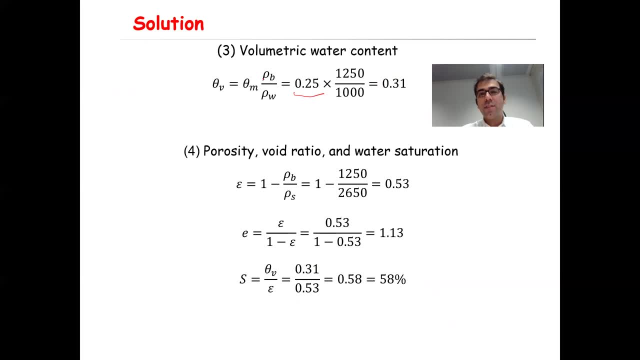 calculated in the first part of this question, which was 25 percent times the bulk density, that is, you calculated in part two, that is 1250, divided by the density of water, which is 1000.. So, and if you do the calculation, you get 0.31 or 31 percent as the